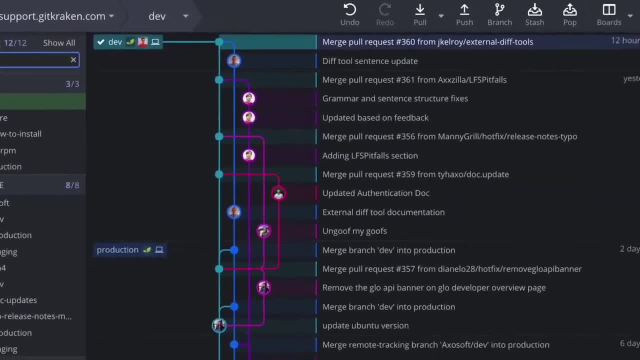 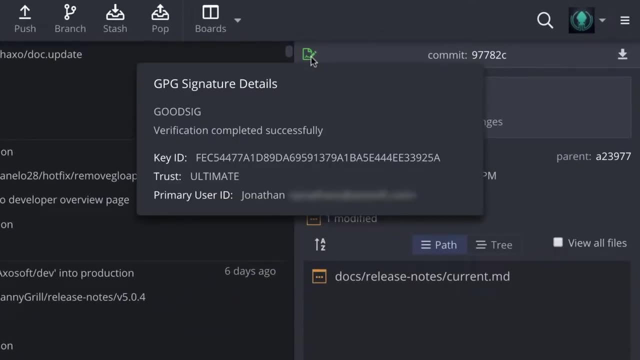 deletion and modification of files and directories that you choose. Basically, you can think of this like a backup for your project, without having to create a bunch of copies at different points in time. Also, these backups are typically stored on cloud servers inside of something called a repository. A repository is 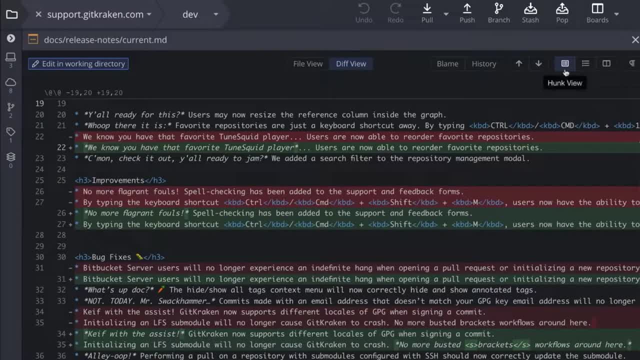 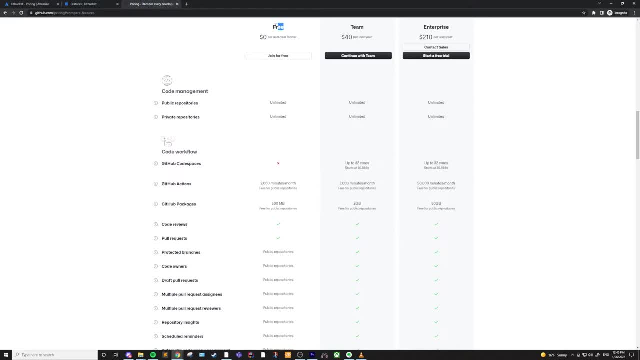 just the history and a collection of all the changes that you've made in one place. This way, you have your backup and you don't have to worry about your hard drive failing and losing everything. Also, most websites will allow you to host repositories for free, Some even give you 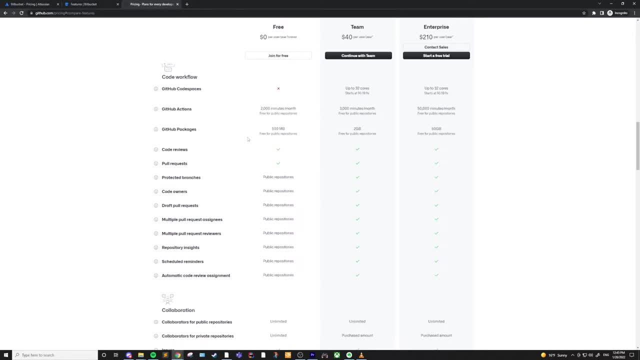 private repositories for free, So there's not really a good reason not to use one. Not only is a VCS a great tool for backups, but it's also invaluable as a collaboration tool. Any software project that has more than one developer maintaining source code files will greatly benefit from utilizing a VCS, Not that. 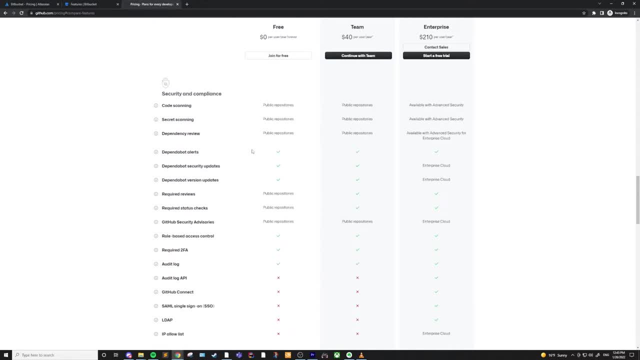 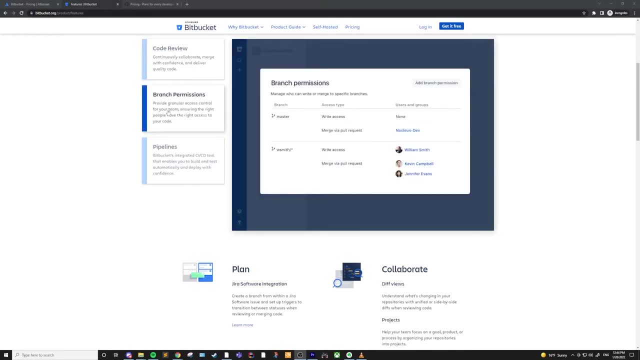 you shouldn't use one if you're a solo developer. I would still say it's completely necessary. There are several collaboration benefits to using a VCS. These include conflict resolution, For example. if you and another person are working on the same project, you can use a VCS to. 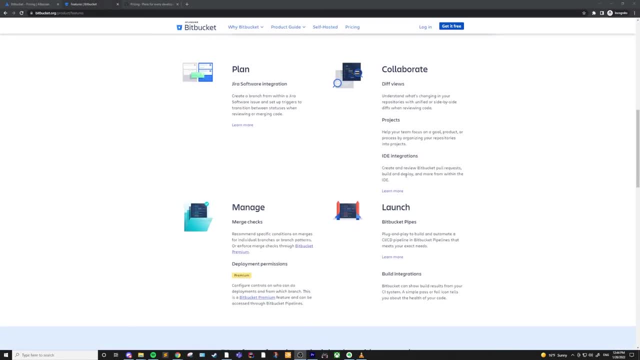 work on the same project and even the same code file at the same time. A VCS will be able to understand that two different people made changes to the same file and it's going to help merge the files so that both people's changes can be in the final file and you don't have to worry about. 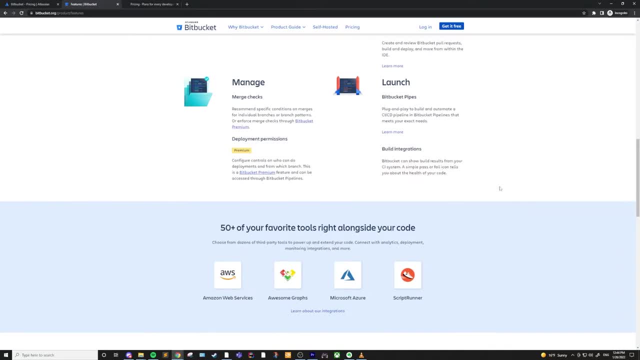 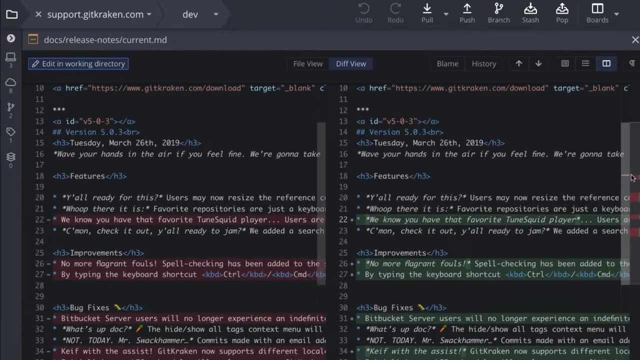 manually copying over changes or one person's changes being lost. A VCS keeps a history of every change to the project, which allows you to roll back and undo changes to source code. So say, you make some code changes and it looks good, but maybe the next day you realize everything is. 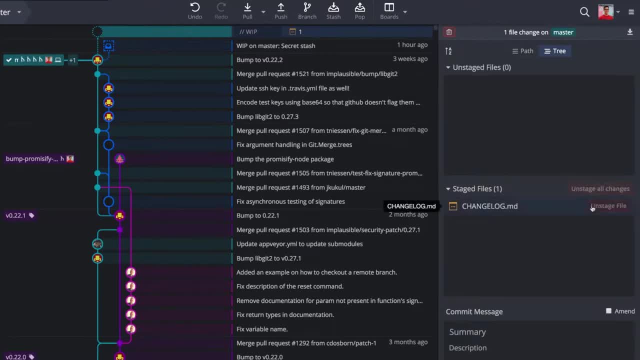 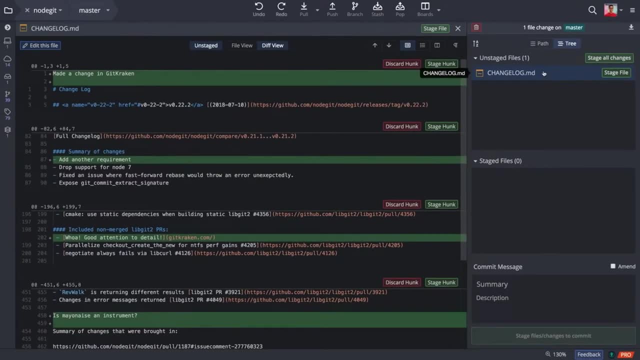 broken With the VCS, you can easily roll back to before those changes and you'll know the exact things that are causing the problem, which helps with debugging and making sure that the software is always in a stable state. Working with a hosted VCS like Bitbucket or GitHub gives you even more. 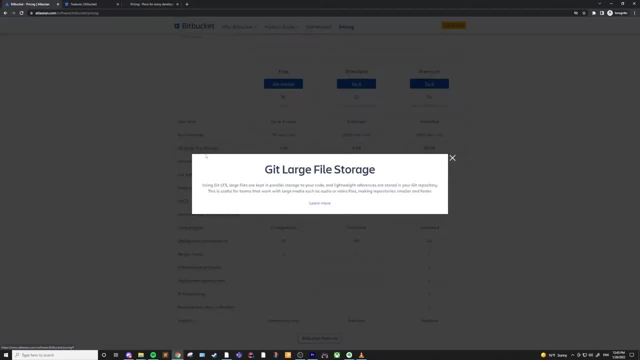 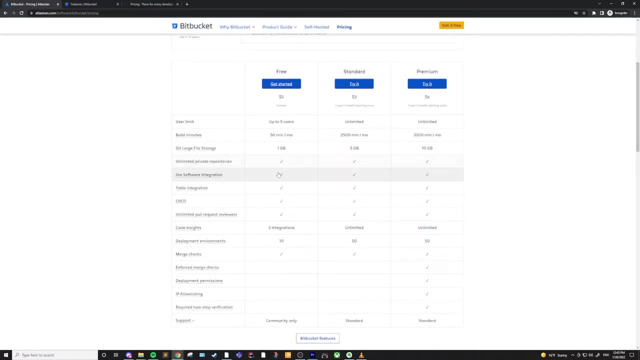 benefits. You can add third-party integrations, For example with Bitbucket. in the past I've used integrations for JIRA task tracking, which can automatically update tasks to some other state, like in review or completed, with a change that I just made and added. or 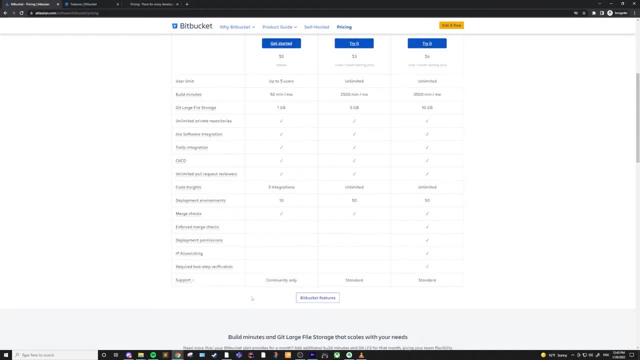 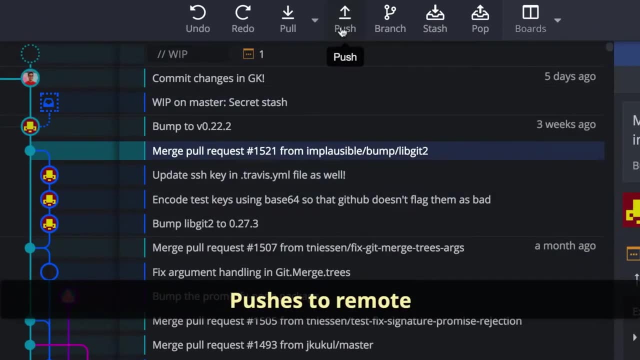 pushed to the repository, And there are dozens of different integrations like this that are going to help with workflow and collaboration. There are many other tools that help facilitate team communication, as well as insight and accountability, since people can see all the changes being made. 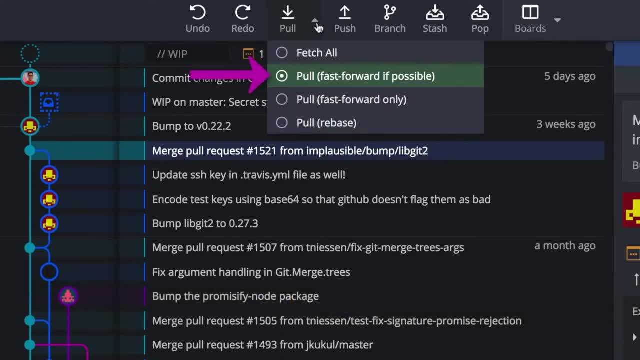 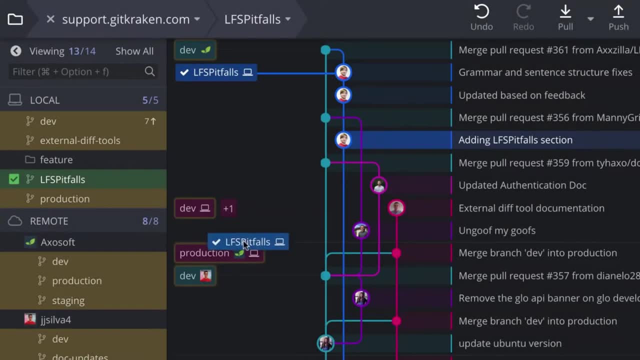 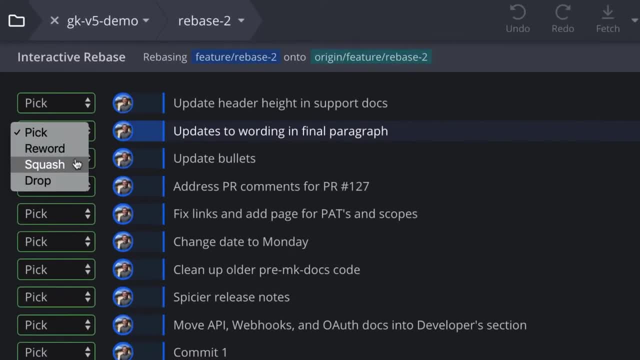 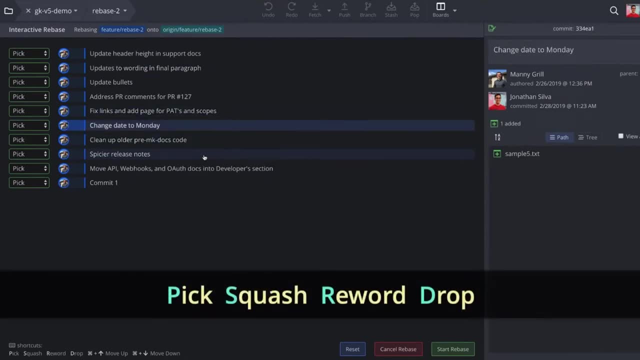 Continuous integration can be set up so that, when a change is added, you can automate a build to start or for tests to start running. This can end up saving you lots of time and effort in the long run. Using a VCS opens up a whole new world to you, and while I could spend hours talking about this topic, 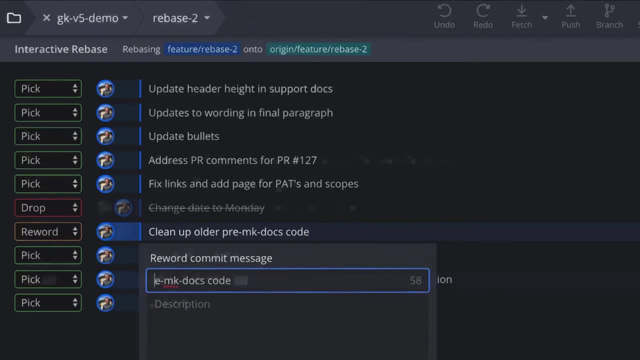 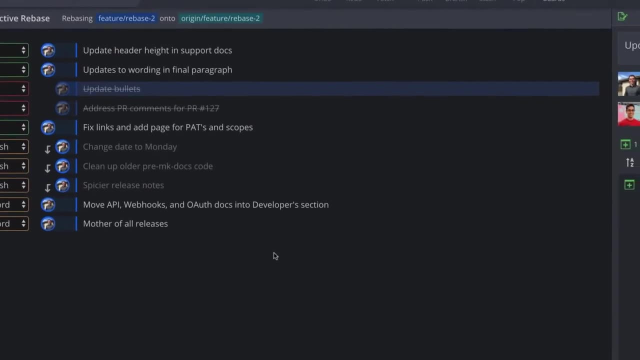 I wanted to give you a quick rundown of what it is and why you should be using it. When I create a new project, this is literally the first thing I do: Create a repository for the project and start using version control. There are many different version control systems and they all have. 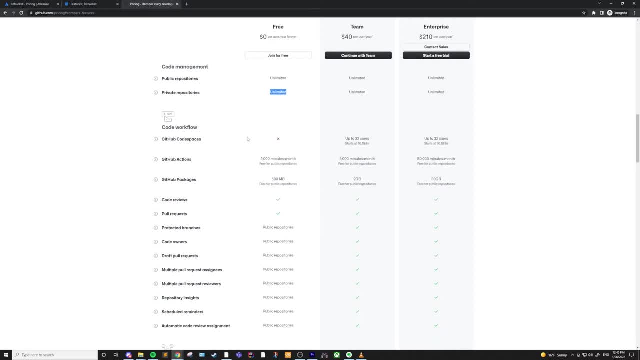 different strengths. There are many different version control systems and they all have. Personally, I use Git and I also enjoy using GitHub and Bitbucket for hosting my repositories and the different integrations that they allow, But, like I said, there are lots of different. 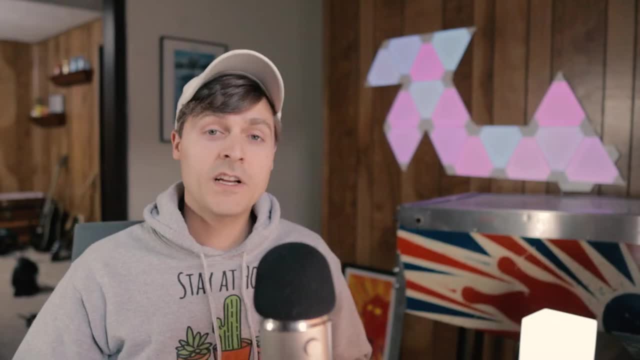 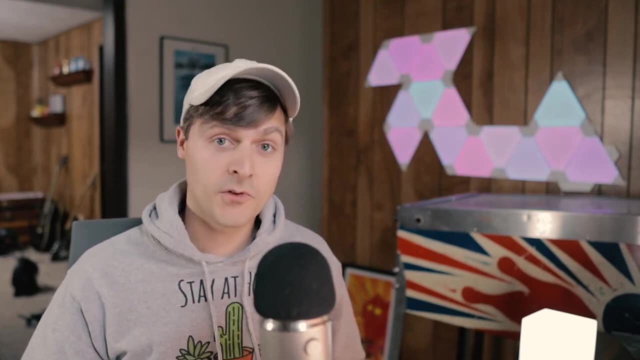 options, so I would try some out and see what you enjoy. Hopefully I helped you understand what version control is and how it can help you. If nothing else, just use it as a backup in case something goes terribly wrong, If you have a story about version control or why you started using it. 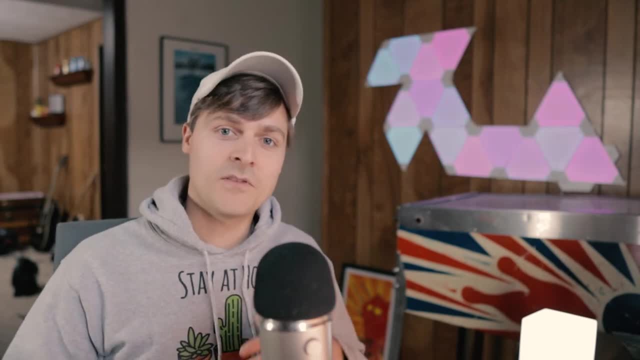 go ahead and leave it in a comment down below. I would love to hear it. If you enjoyed the video, please subscribe to my channel and I'll see you in the next one. Please leave a thumbs up If you want to see more content like this in the future. 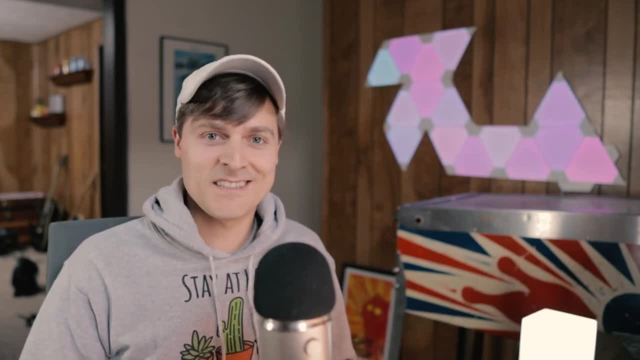 go ahead and subscribe, As always. have fun creating and I'll see you next time.